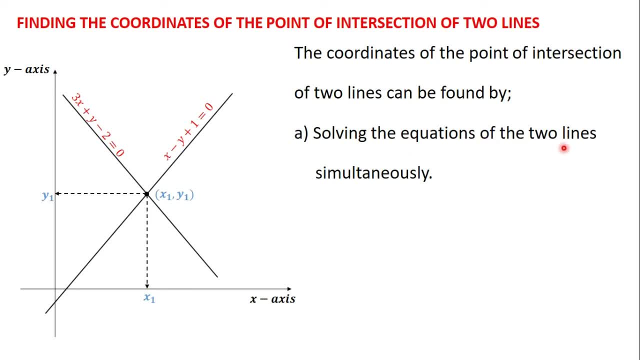 can be found by a Solving the equations of the two lines simultaneously. So when you have the equation of the first line and the equation of the second line and you want to find the coordinates, the point of intersection of those two lines, you have two options. the first option is that you 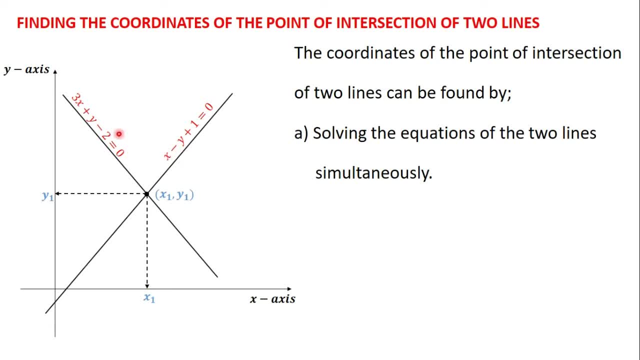 solve the two equations that you have simultaneously. so if you solve this equation and that equation simultaneously, you are going to get values for x and y. the x value will give us the s coordinate of the point of intersection of the two lines, and the y value will give us the y coordinate of the. 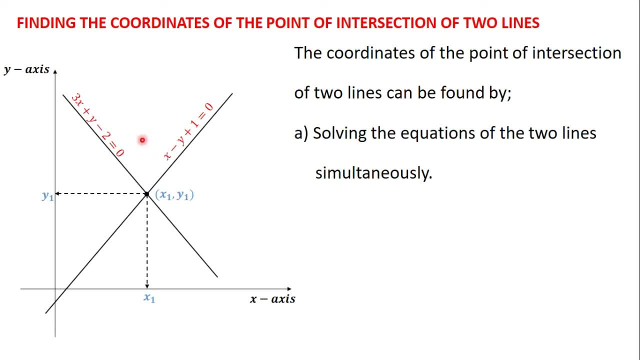 point of intersection of the two lines. so when you are given the equation of the two lines, you can find the coordinates of the point of intersection by one, solving the two equations simultaneously. another option is by graphing the equations of the two lines. this means that you are 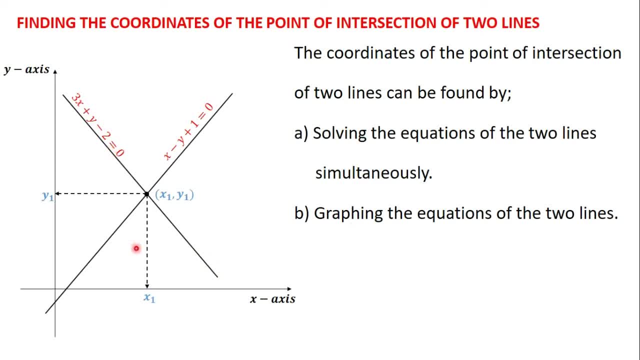 going to draw the graph of the first equation and you draw the graph of the second equation on the same graph sheet. now, when you draw the graph of the two equations on the same graph sheet, you will see that they will meet as a certain point. 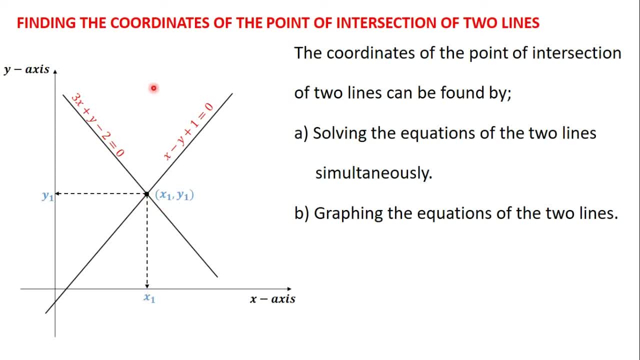 When you trace that point to the x-axis, you will get the x-coordinate of the point of intersection, and when you trace it to the y-axis you will get the y-coordinate of the point of intersection. So when you are given the equation of two straight lines, you can find the coordinates. 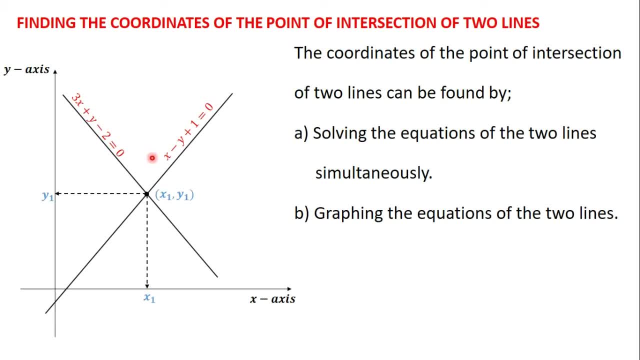 of their point of intersection by solving the equations of the two lines simultaneously, or two graphing the equations of the two lines. So, for example, if you want to find the coordinates of the point of intersection of the two lines that we have in our diagram, that is, if you want to find the coordinates of the point, 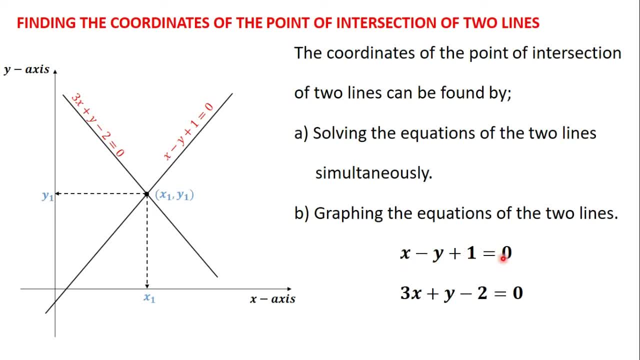 of intersection of the line x minus y plus one is equal to zero, and the line three, x plus y minus two, is equal to zero. we can solve these two equations simultaneously for the values of x and y, Or we can draw the graphs of the two lines on the same graph sheet and then from the graph